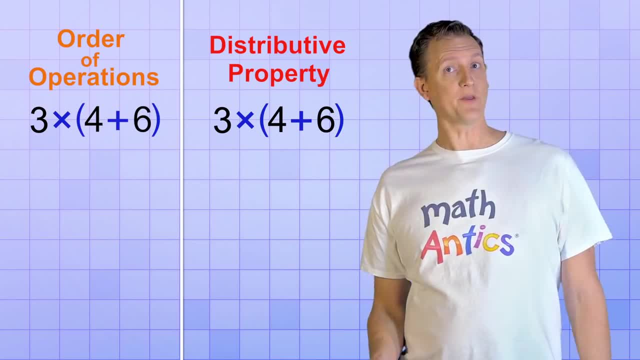 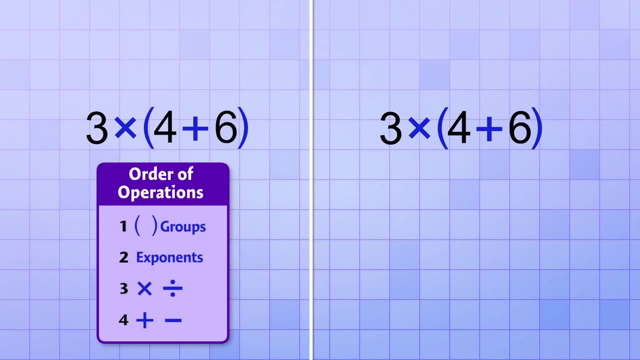 But the second way will use the Distributive Property And if we do the arithmetic right, both ways will give us the same answer. So for the first way, our order of operations rules tell us that we need to do any operations inside of groups first. 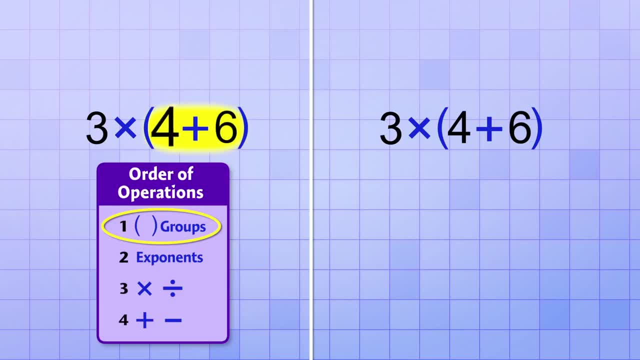 And since these parentheses form a group, we first need to add the 4 and 6, which gives us 10.. Next we can multiply that by 3, which gives us the final answer of 30.. Now let's use the Distributive Property. 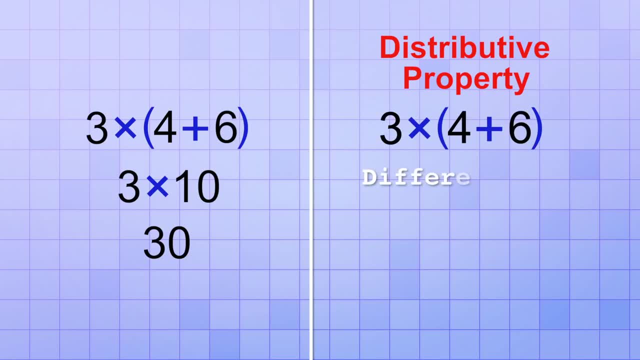 The Distributive Property allows us to change this expression into a different form. Instead of multiplying 3 by the whole group at once, we can distribute that factor of 3 and multiply it by each member of the group individually. That means we'll make a copy of the 3 times for each member of the group, the 4 and the 6.. 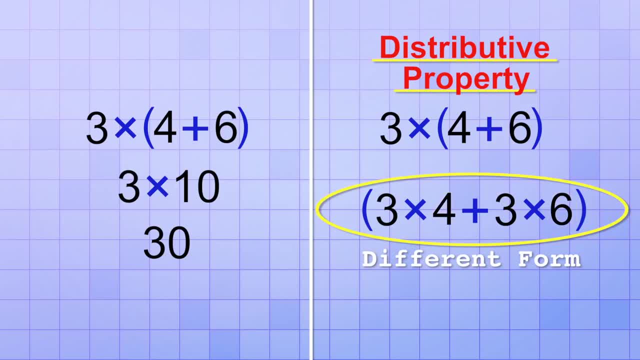 So, after applying the Distributive Property, our expression looks like this: 3 times 4 plus 3 times 6.. Because we distributed the multiplication to each member of the group, the group isn't needed anymore, so the parentheses can go away. 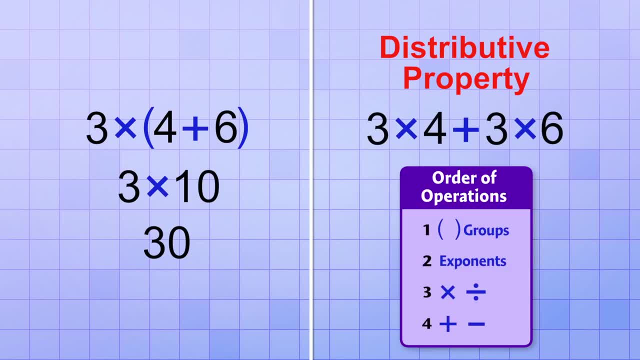 Now we can continue to simplify this new form using our order of operations rules. Those rules tell us to do multiplication before addition. So 3 times 4 is 12 and 3 times 6 is 18.. The last step is to add those two results together. 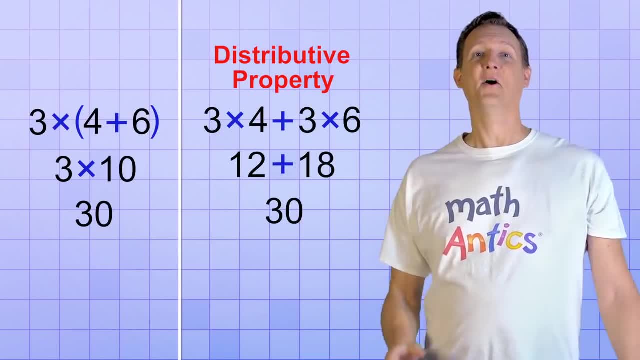 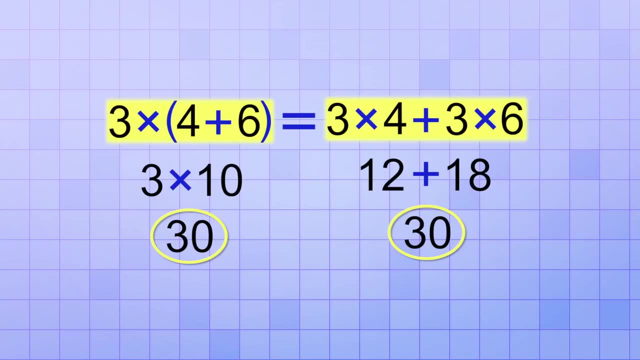 12 plus 18 equals 30. Well, look at that. We got the same answer in both cases, which means our original expressions are equivalent, even though they have different forms. In the first form, the factor 3 is being multiplied by the entire group all at once, so we needed to do the addition inside that group first. 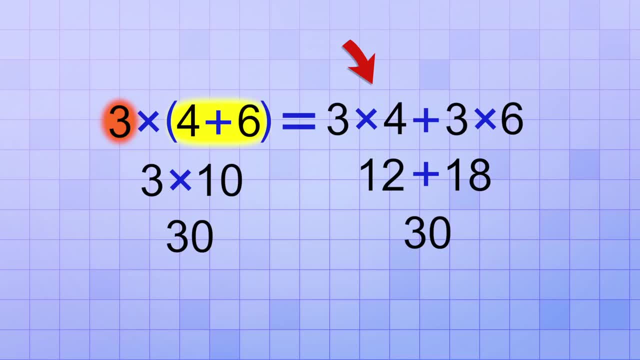 But in the second form we used the Distributive Property to rearrange the expression so that the factor of 3 is multiplied by each member of the group individually instead of the whole group all at once. Distributing that factor made the group go away. 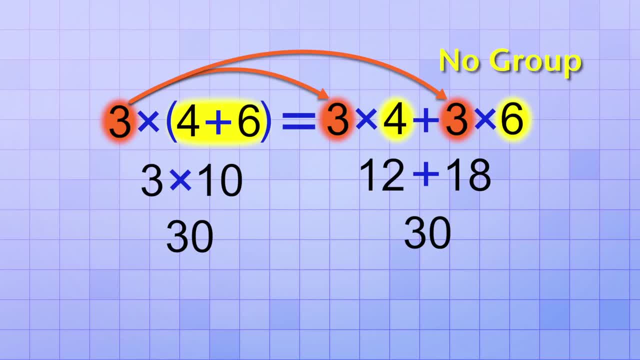 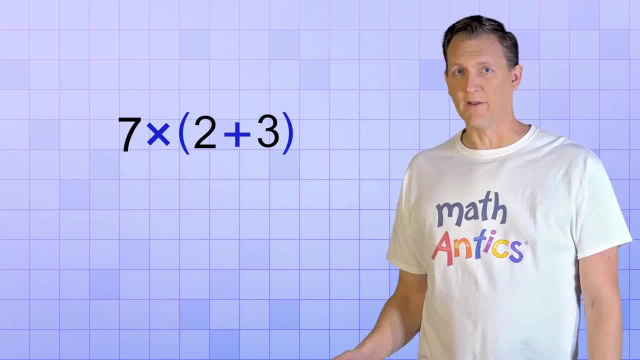 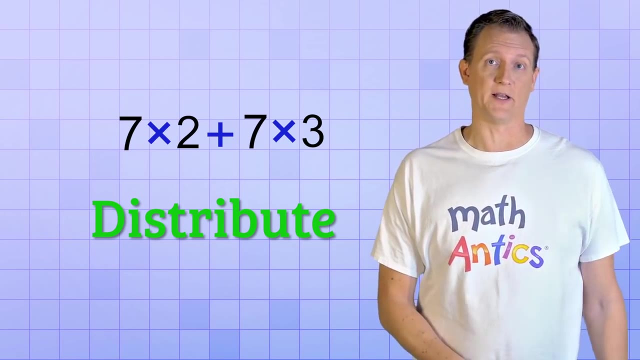 So we didn't have to do the addition inside that group first. So the Distributive Property is basically a way of getting rid of a group that is being multiplied by a factor. If you distribute the factor to each member of the group, you'll get the same answer. you would if you calculate what's in the group first and then multiply. 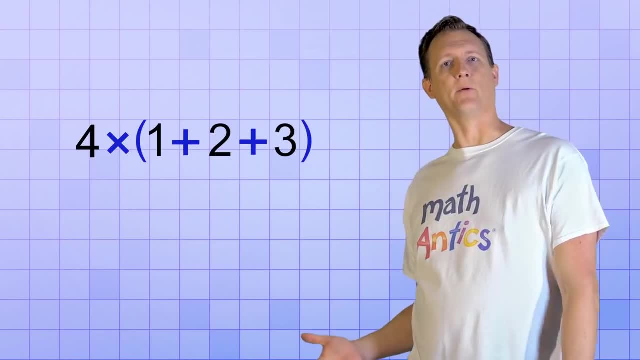 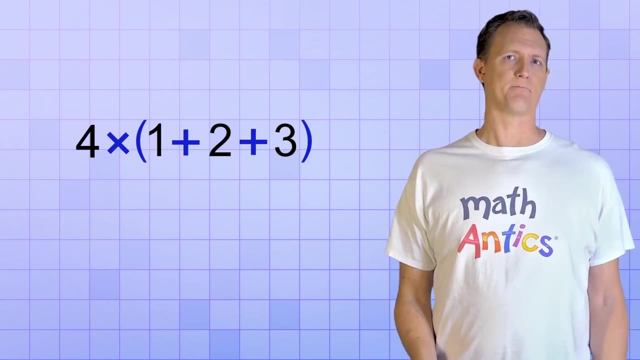 And it works no matter how many members are in the group. Like in this problem, we have to multiply 4 by the group, 1 plus 2 plus 3.. Again, let's try simplifying this both ways. In the first way, we start by simplifying what's in the group. 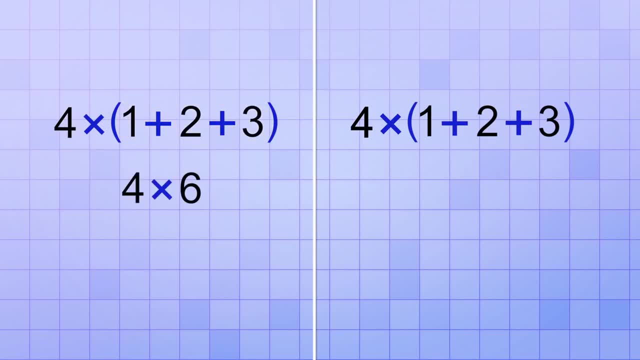 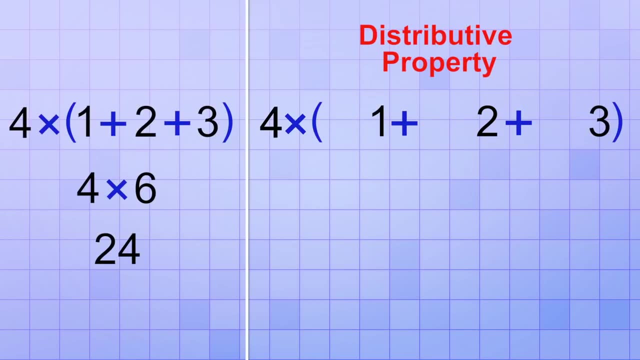 1 plus 2 plus 3 equals 6.. And then we multiply 4 times 6,, which gives us 24.. Now let's use the Distributive Property. We distribute a factor of 4 to each member of the group, which makes the group go away and allows us to do those multiplications individually. 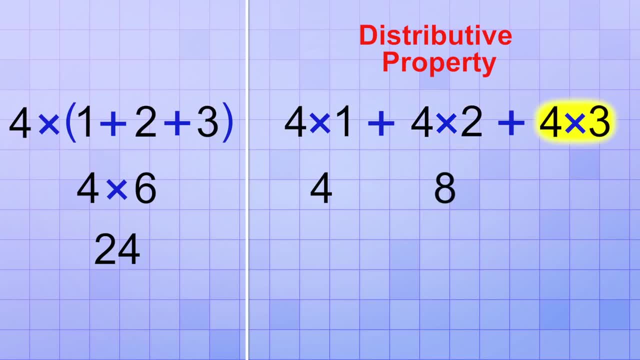 4 times 1 is 4.. 4 times 2 is 8. And 4 times 3 is 12.. Finally, we add up those three individual answers: 4 plus 8 is 12. And 12 plus 12 is 24.. 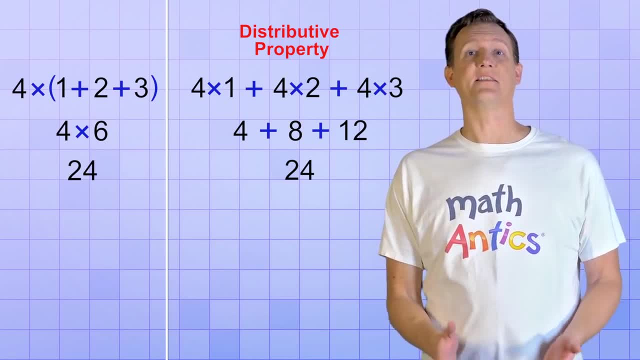 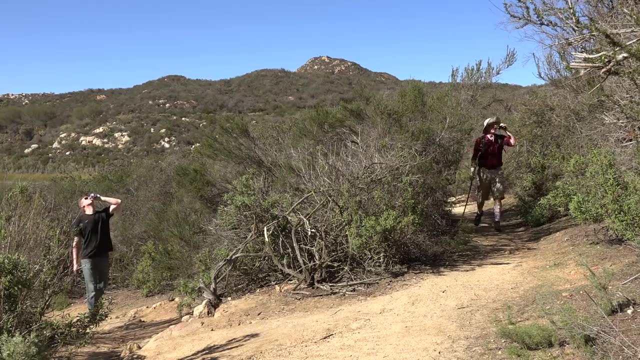 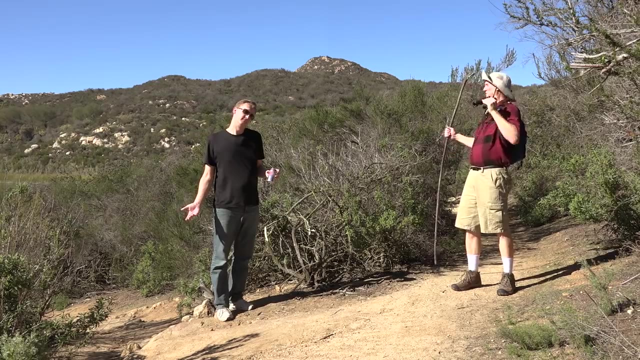 See, The Distributive Property gave us another way to arrive at the same answer. It's like the Distributive Property is an alternate path that you can take to arrive at the same point. What are you doing here? I'm always here, Okay, great. 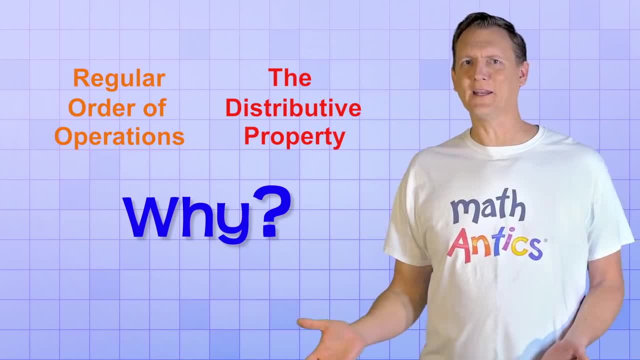 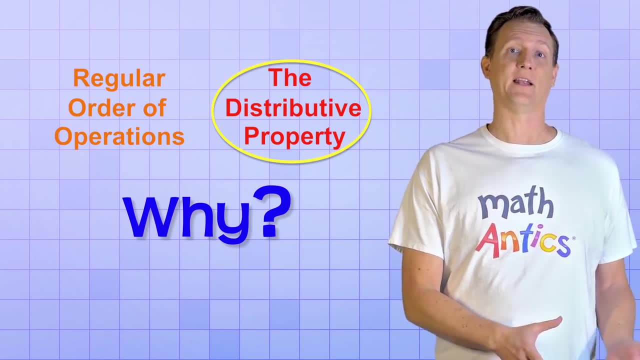 We have two ways to get to the same answer, But why do we need two different ways to do this? Why do we need two different ways to do the same calculation? And it seemed like the Distributive Property way was even more complicated than the regular way. 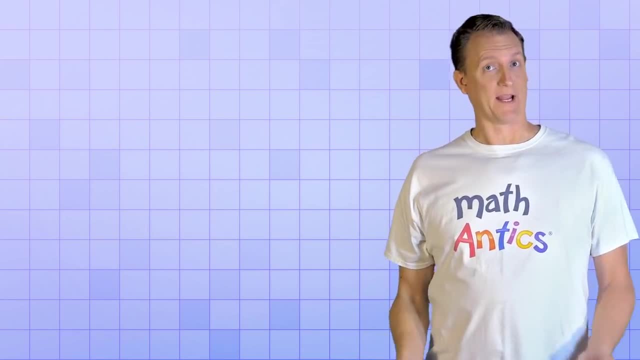 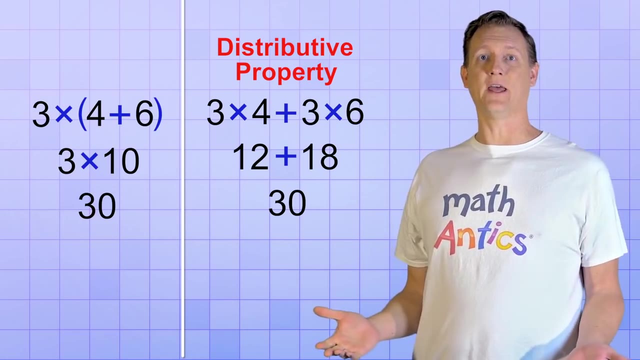 Why would we ever want to use it? That's a good question And it's true. There are times when the Distributive Property way is harder, like in our first problem. It was easier to just go ahead and simplify the group first, because it's easy to multiply 3 times 10 mentally. 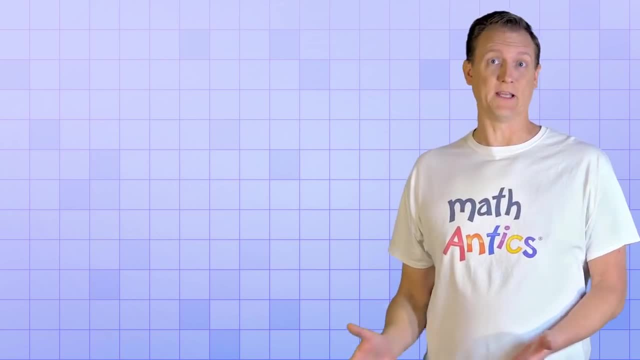 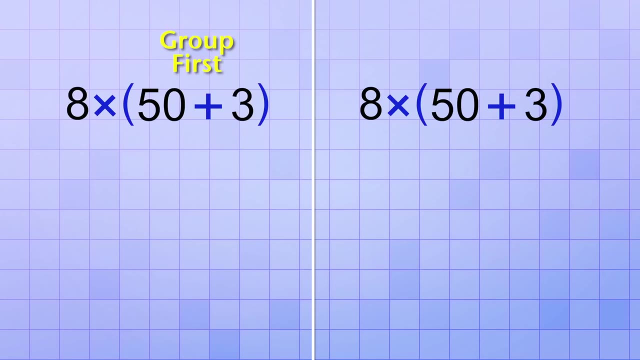 But there are also times when the Distributive Property way is easier, like in this case, 8 times the group. If we decide to simplify the group first in this problem, we end up needing to multiply 8 times 53. But if we apply the Distributive Property instead, 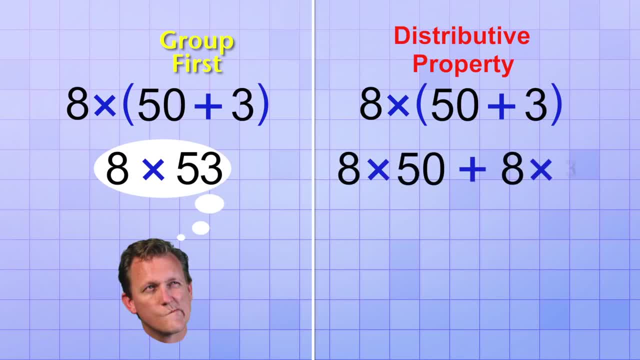 we can change the expression into- and that's easier to do mentally: 8 times 50 is 400 and 8 times 3 is 24, so the answer is 424.. Realizing that the Distributive Property can make us really lazy and fuss. 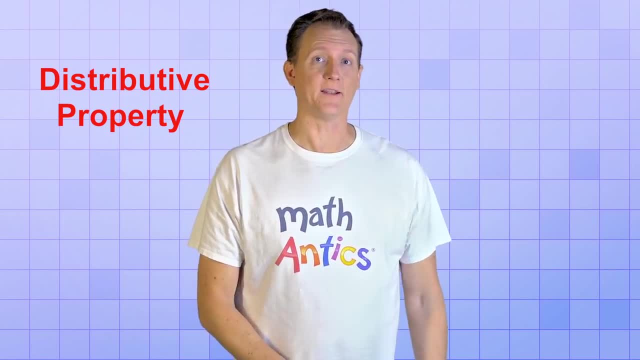 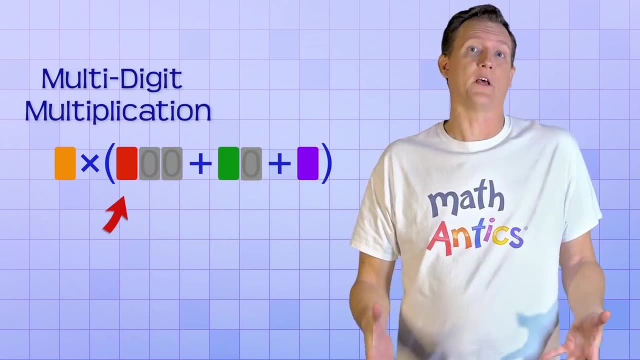 What makes sum calculations easier to do mentally can come in really handy for certain basic multi-digit multiplication problems. That's because you can break up the multi-digit factor into a group sum you know like expanded form, and then distribute the other factor to the members of that group. 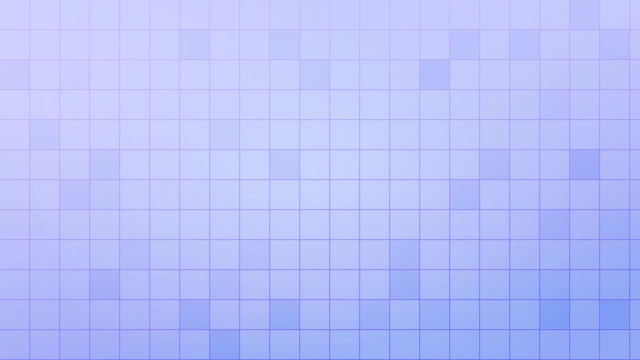 Sound confusing. Here's what I mean. Let's say you need to multiply 5 times 47. Well, you could just use the multi-digit multiplication procedure, or you could change this into a problem where the distributive property will make it a little easier to do. 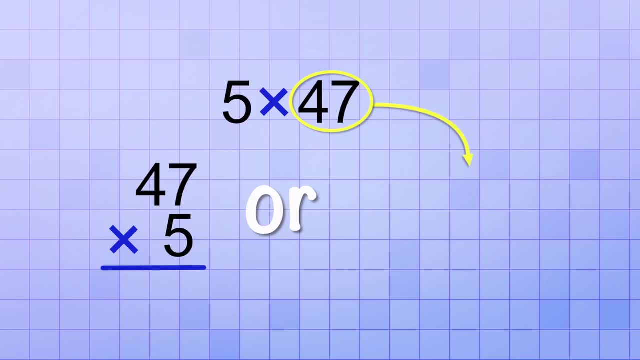 The key is to realize that you can replace the 47 with 40 plus 7.. Then the problem becomes 5 times the group 40 plus 7.. And the distributive property lets us change that into 5 times 40 plus 5 times 7.. 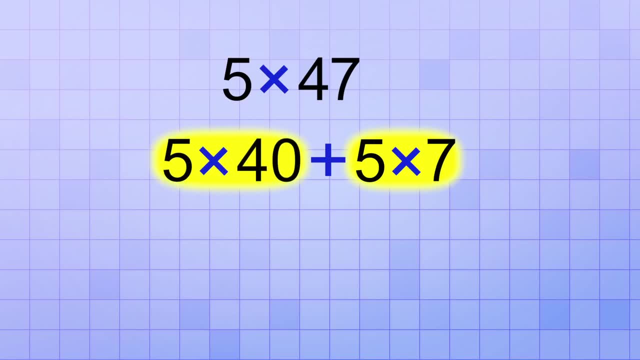 Those two multiplications are easy to do: 5 times 40 is 200 and 5 times 7 is 35. So our answer is 200 plus 35.. Want to see another example? Let's apply that same idea to this multiplication problem. 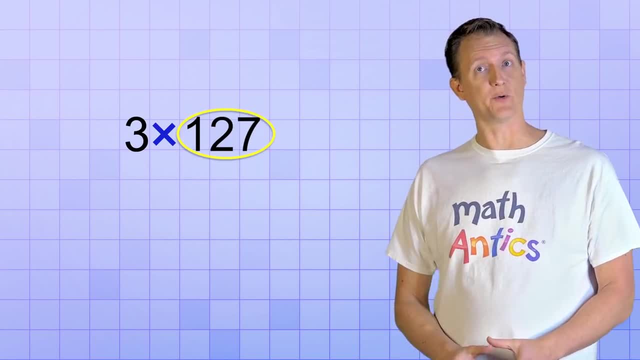 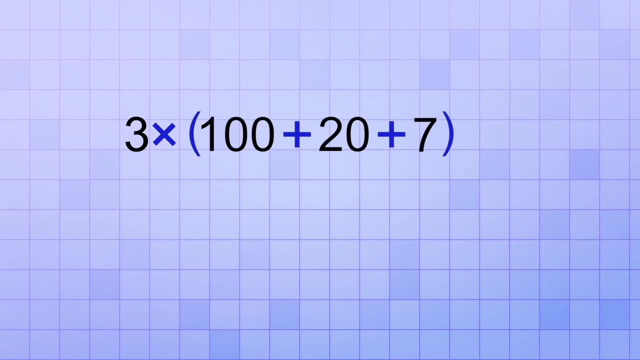 3 times 127. But instead of 127, let's change that into the group 100 plus 20 plus 7.. We need to multiply that by 3 and the distributive property lets us distribute that multiplication to each member of the group. 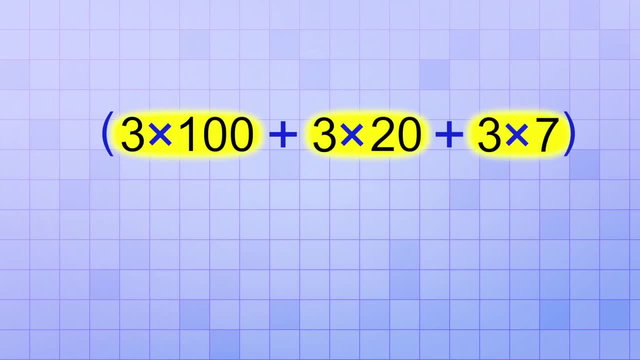 3 times 100 plus 3 times 20 plus 3 times 7.. That helps because we can do those mentally. 3 times 100 is 300.. 3 times 20 is 60. And 3 times 7 is 21.. 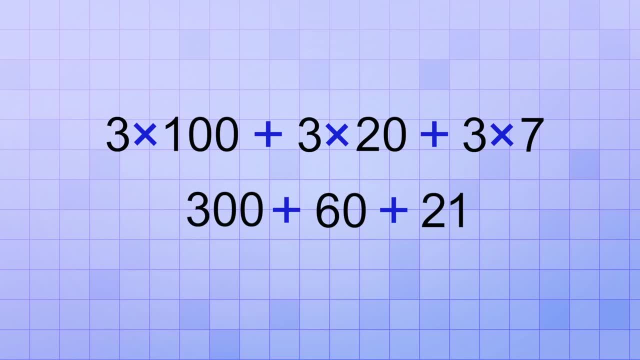 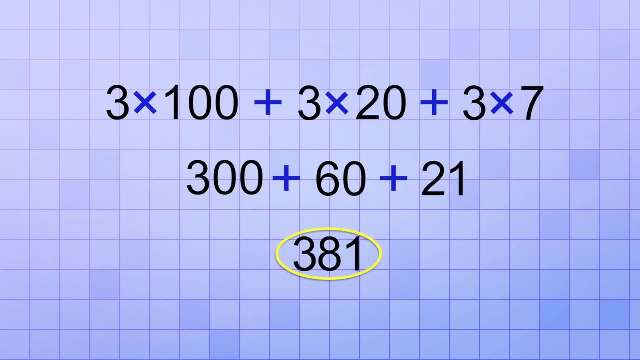 All that's left to do is add those three products up, which is not too hard to do mentally either. 300 plus 60 plus 21 gives us 381 as our final answer. Now, before we wrap up, there's one more important thing that you should know about the distributive property. 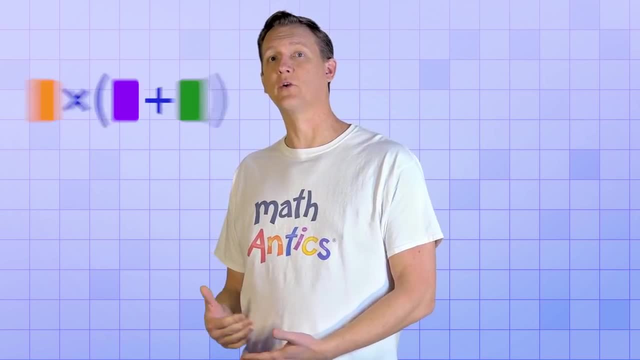 You already know that the distributive property works when the members of a group. you already know that the distributive property works when the members of a group. you already know that the distributive property works when the members of a group are being added. 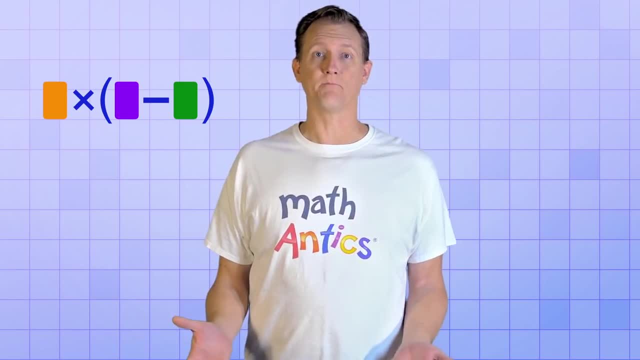 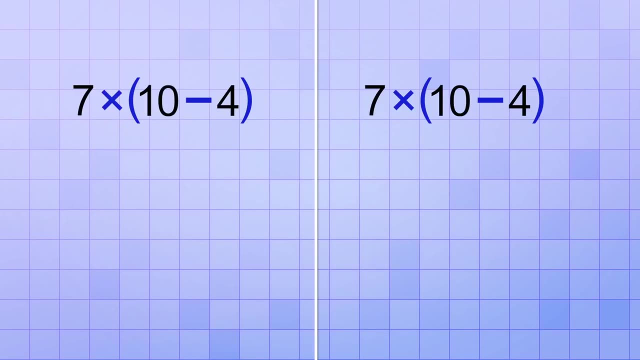 But it works the same way for members of a group that are being subtracted, Like in this problem, seven times the group, ten minus four. You could do this problem the typical way and simplify the group first. Ten minus four is 6.. 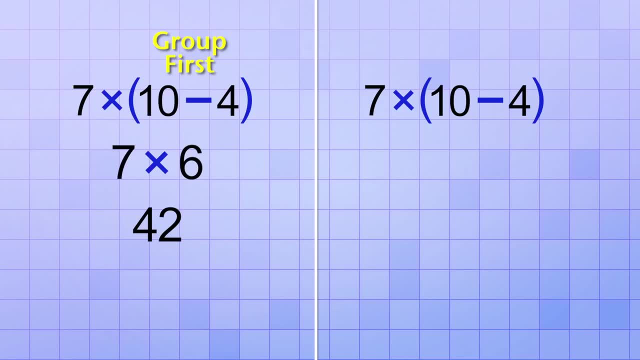 And then 7 times 6 gives us 42. Or you could use the distributive property. You distribute the seven times to both members of the group to get 7 times 10 minus 7 times 4.. 7 times 10.. 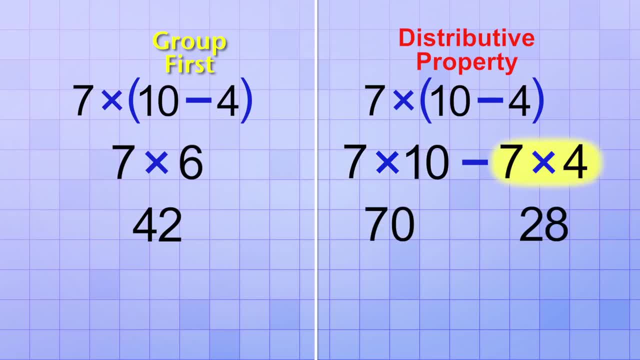 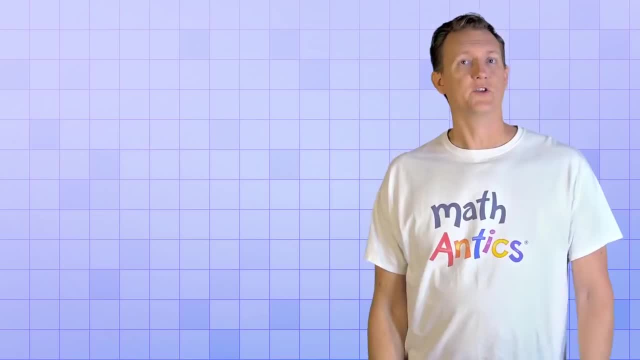 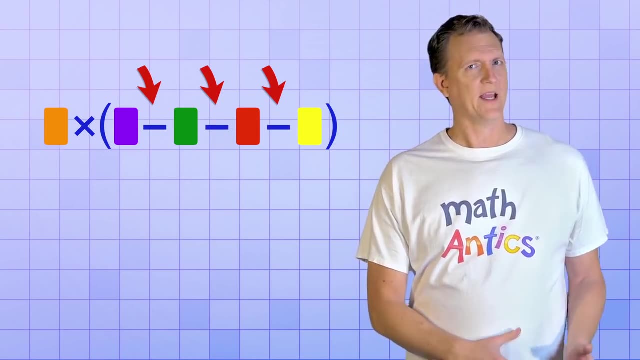 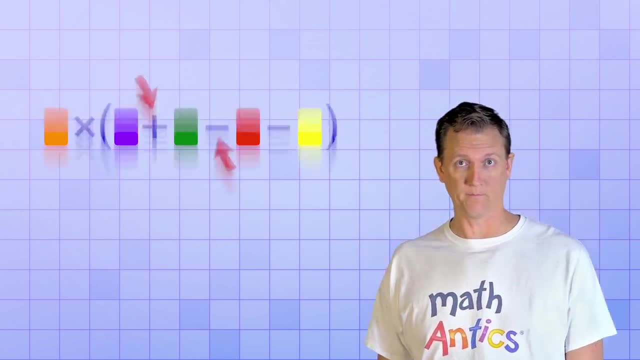 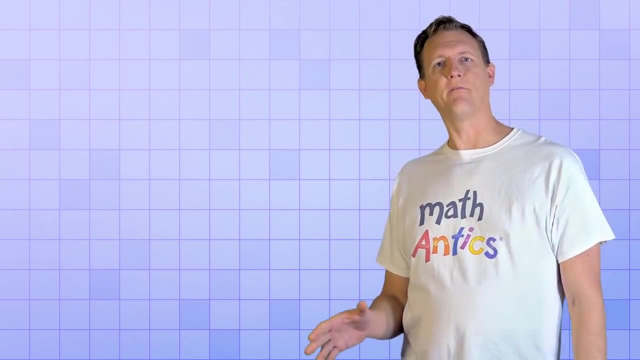 even if there's a mixture of addition and subtraction in the group, But the Distributive Property doesn't work when the members of a group are being multiplied or divided. For example, if you have 5 times the group, 2 times 3,. 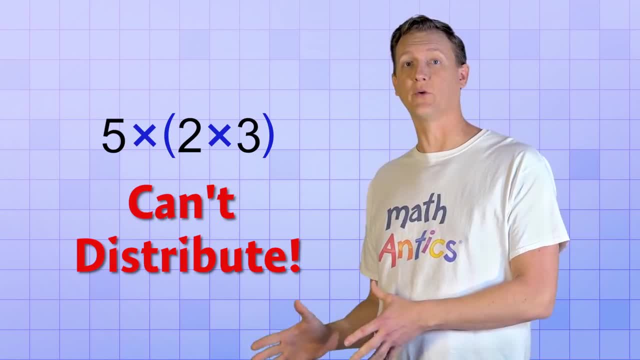 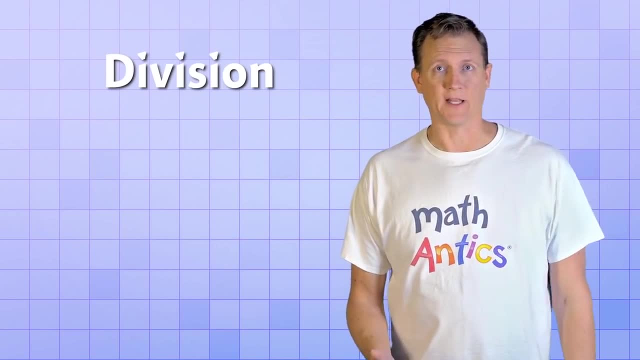 you CAN'T distribute a copy of the factor 5 to each member of the group without getting a completely different answer, And the same goes for division, If the members of a group are being divided like 4 times the group, 6 divided by 2,. 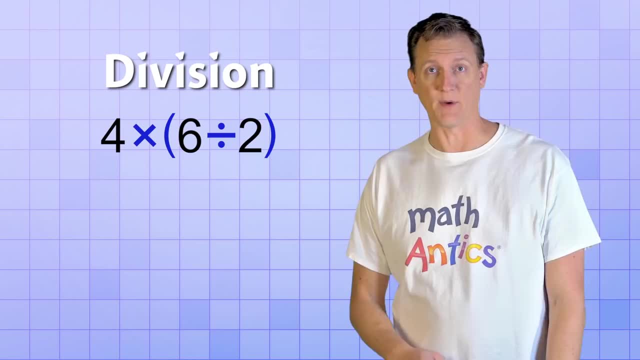 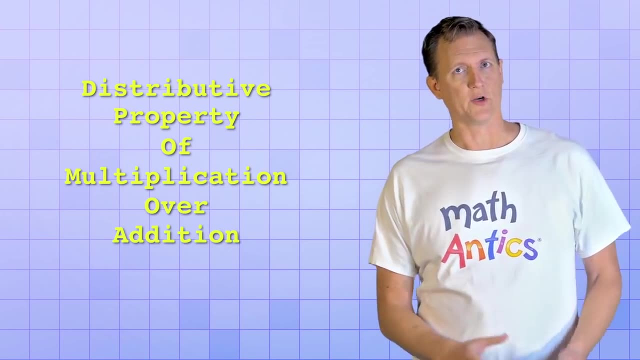 you will NOT get the right answer if you distribute the factor 4 to each member. That's why the technical name is the Distributive Property of Multiplication over Addition. You're distributing the multiplication over all of the members of a group that are being added. 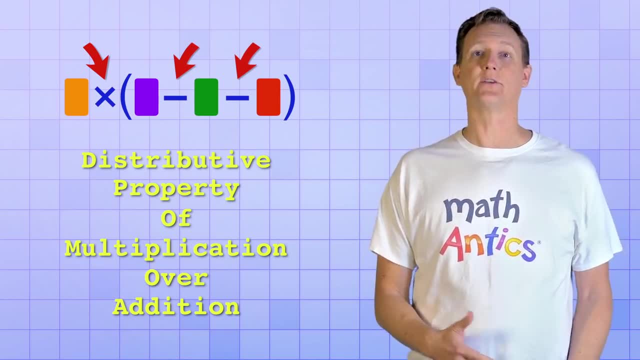 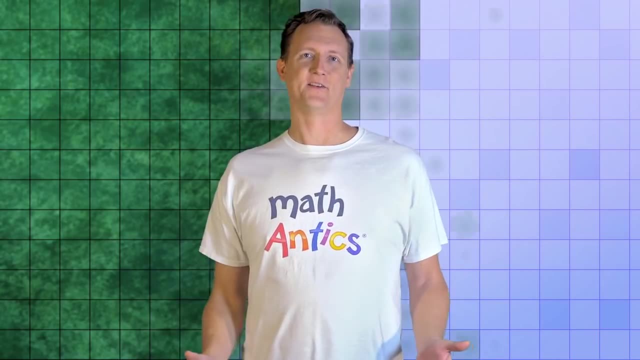 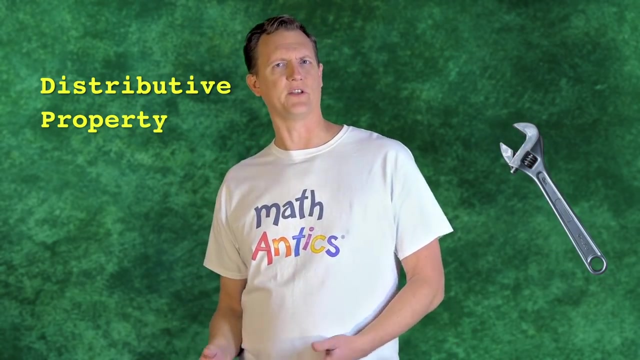 And the reason that it also works for subtraction is that subtraction is really just a negative form of addition, since subtraction and addition are inverse operations. Alright, so the Distributive Property is a handy way to rearrange arithmetic expressions. It's like a tool that you can use in certain situations if you think it will make a particular calculation easier to do. 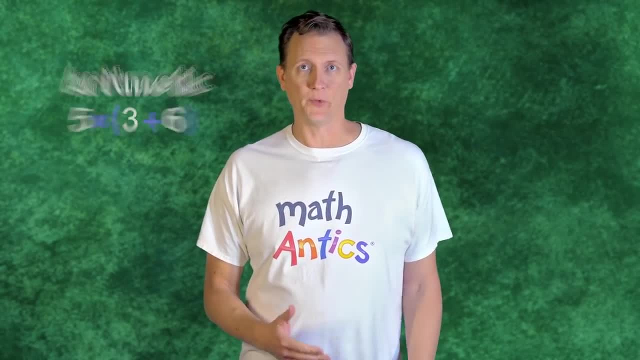 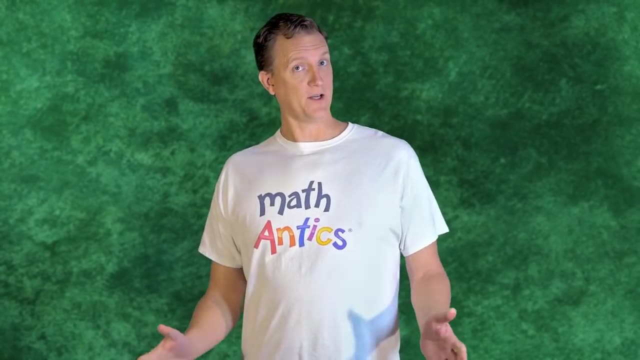 And even if you don't end up using the Distributive Property a whole lot for arithmetic, it's still a really important math concept that will be even more useful when you get to Algebra. Until then, be sure to practice what you've learned in this video by trying some of the exercise problems. 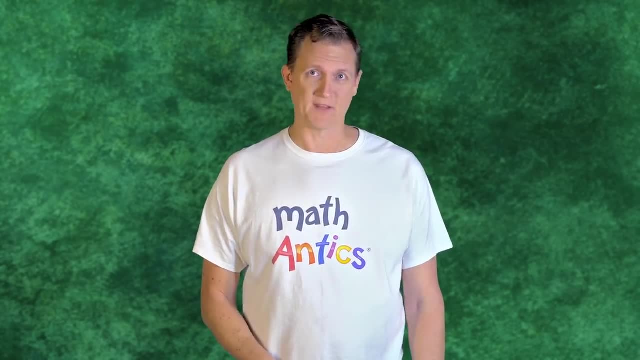 Practice is the best way to make sure that you really understand. As always, thanks for watching Math Antics and I'll see you next time. Learn more at wwwmathanticscom.